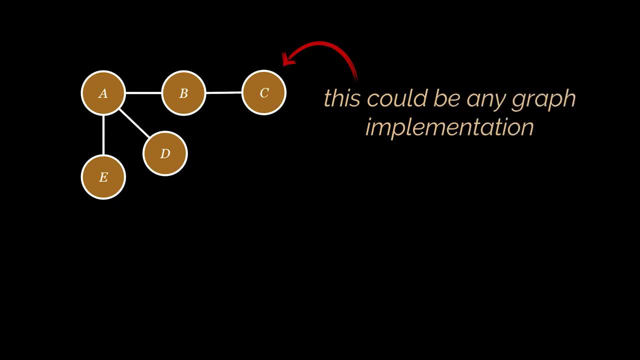 or rather you don't want to expose the underlying implementation of this graph. Maybe this graph is a binary search tree or a red black tree, Why care, Just like the guide doesn't really know who you are, but still is able to help you. All you want is to traverse the elements of this graph. 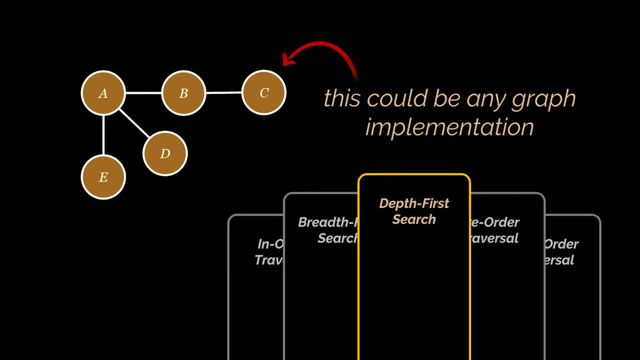 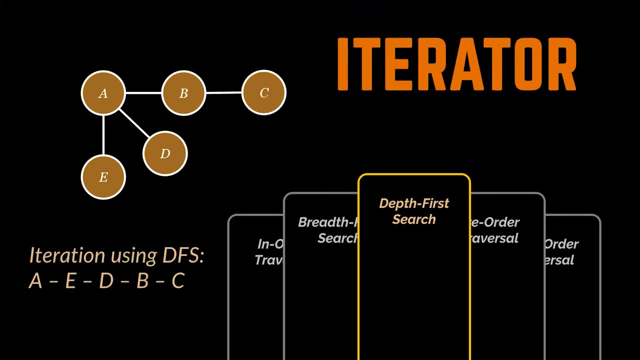 in a depth, first touch manner, let's say, Or in our example, all we want is to visit these particular sites that we find interesting, And to do that, the guide we hired will tailor the tour according to our liking. Or, similarly, the iterator will visit the elements of the graph according to the algorithm we picked. 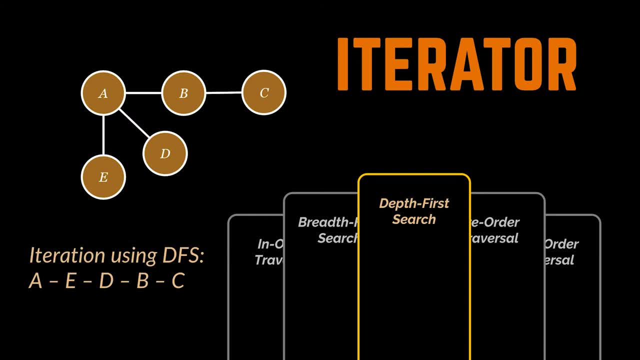 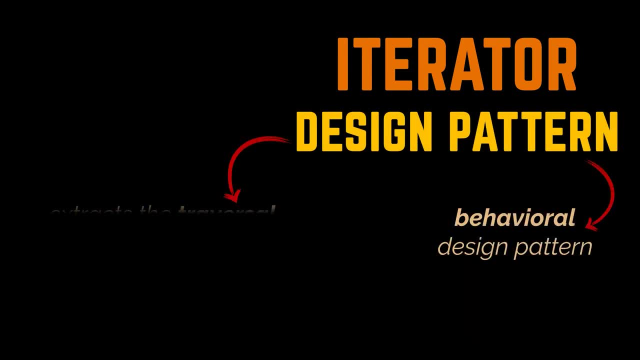 and regardless of the actual underlying implementation of this graph. So the iterator design pattern is a behavioral design pattern which main idea is to extract the traversal behavior behavior of a collection into a separate object called an iterator. This iterator object, on top of providing a way to traverse the elements of a collection, 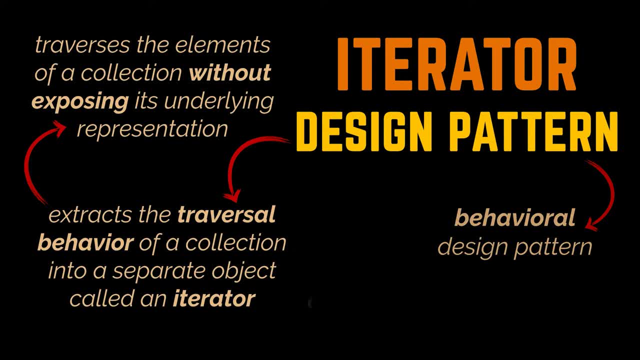 without exposing its underlying representation, encapsulates all of the traversal details, such as the current position and how many elements are left till the end. Because of this, several iterators can go through the same collection at the same time, independently of one another. 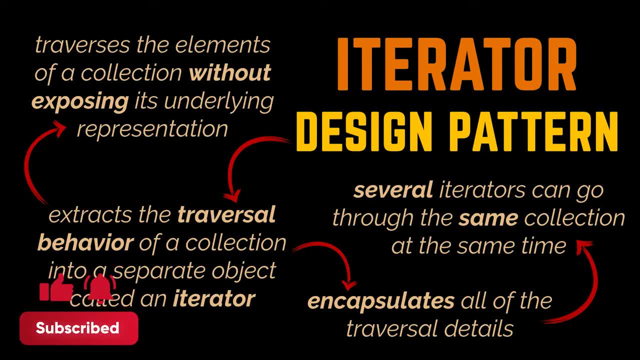 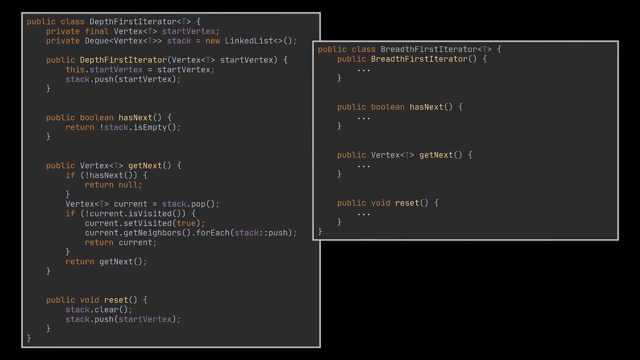 Now, if you have been watching our videos, you should be familiar with the example we are about to implement using the iterator pattern. This example will consist of two classes: the depth first- iterator, and the breadth first, iterator. classes you can see in front of you. 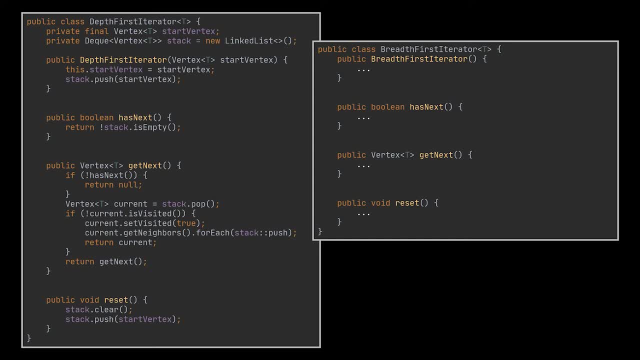 Now I am not going to dive in the details of their implementation, as both of them were already covered in previous videos and because I want the iterator pattern itself to be the main focus of the video, not the traversal algorithms. All I did here was kind of adapted these implementations. 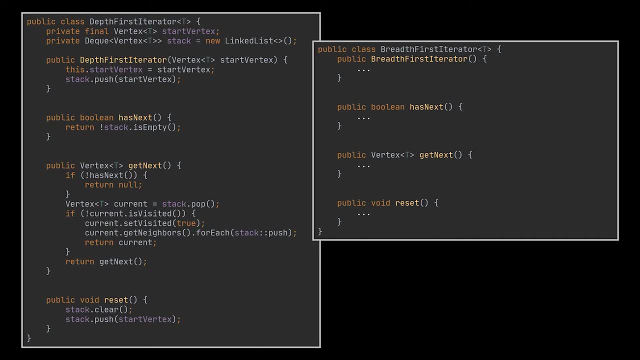 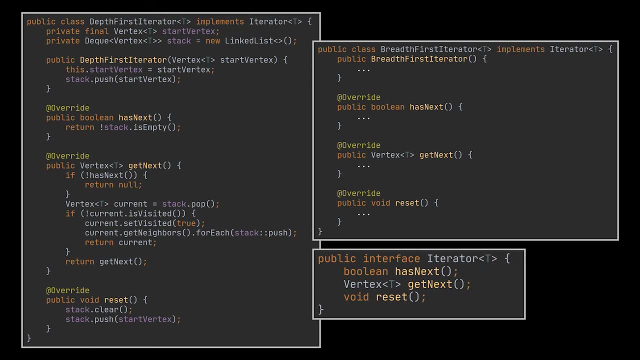 Ok, the last missing piece is the interface. All iterators must implement the same interface. This makes the client code compatible with any collection type or any traversal algorithm. If you want to introduce a new way of traversal, you just create a new iterator class. 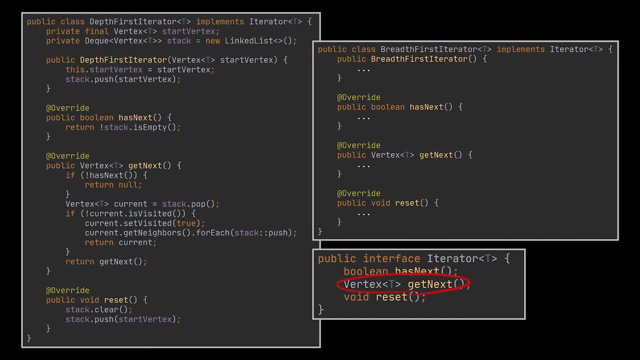 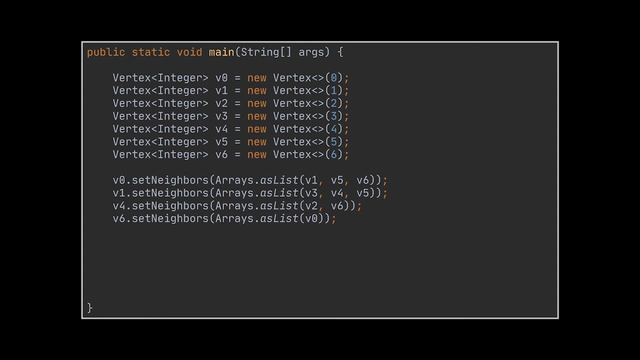 Usually, iterators must at least provide one primary method for fetching the elements of the given collection. The client can keep running this method until it returns true. It returns null, which means that the iterator has traversed all of the elements. Now to test our code, all we have to do is create a bunch of vertices, assign their corresponding 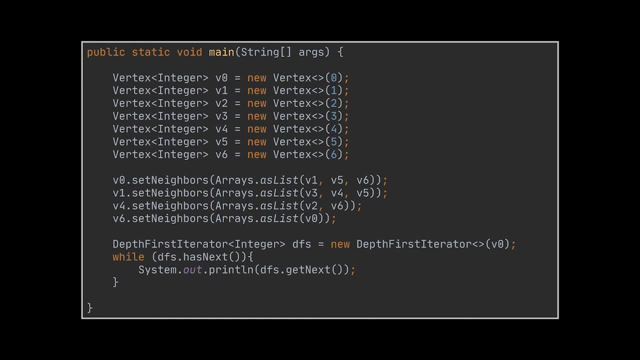 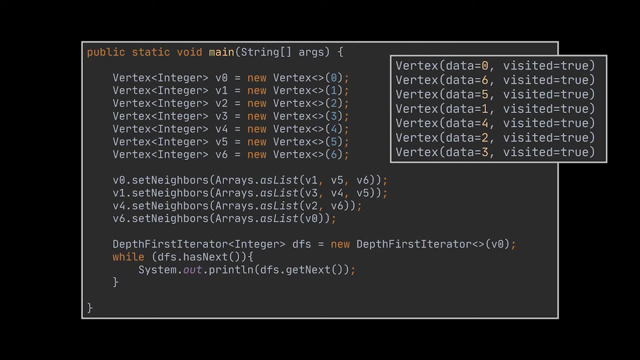 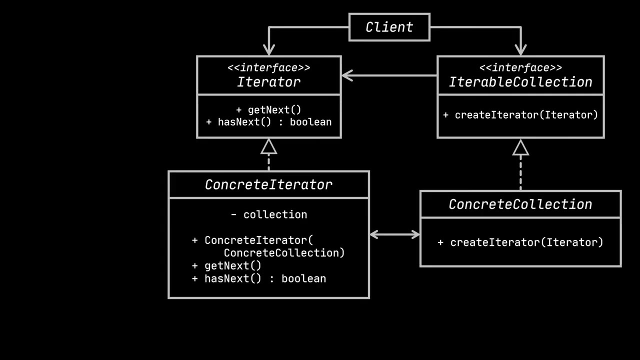 neighbors, then pick the iterator we want to use and invoke the methods we just implemented. When we run this piece of code, you can see that the output we obtain is a depth first search traversal, as expected. Let's go ahead now and take a look at the structure or class diagram of the iterator. 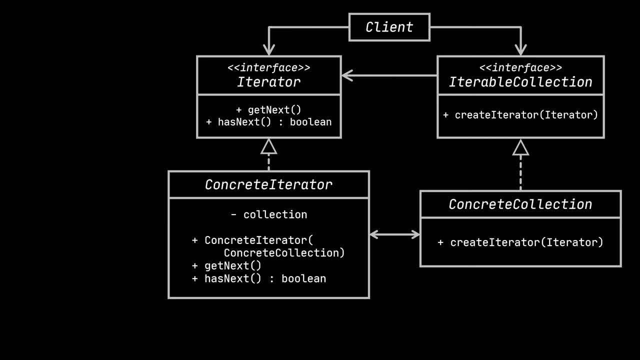 design pattern. Taking it to the graph traversal example we just implemented, The first thing you may have noticed is the iterator interface. The iterator interface declares the operations required for traversing a given collection, like fetching the next available element or retrieving the current one, etc. 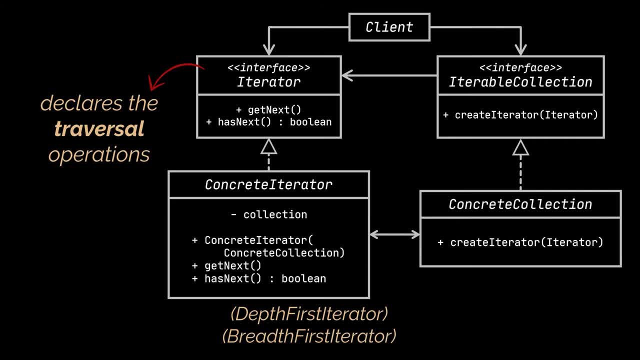 Next are the concrete iterators, which were represented by the depth first iterator and the breadth first iterator classes in our previous example. Before traversing a given collection, the iterator object should track the traversal progress on its own. This allows several iterators to traverse the same collection independently of each. 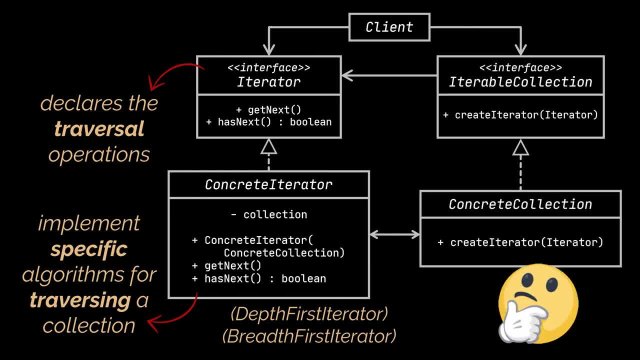 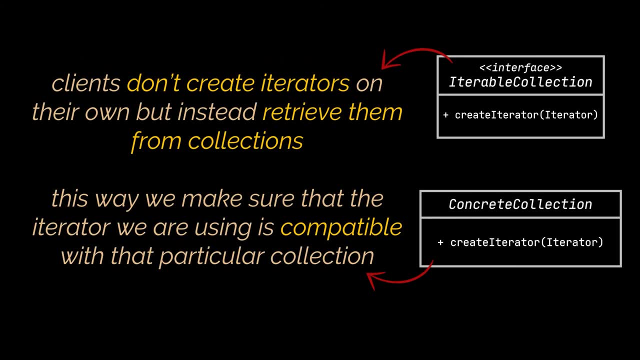 other. Okay, the remaining pieces of this diagram are the collection interface and the concrete collections. And you may be thinking that in the traversal example we implemented, we didn't have matching classes for these, And you are right. You see, usually clients don't create iterators on their own like we did. 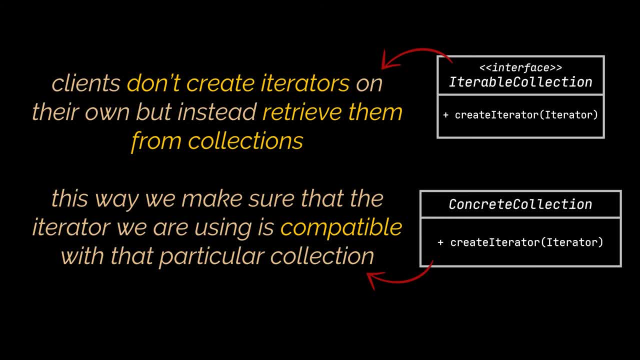 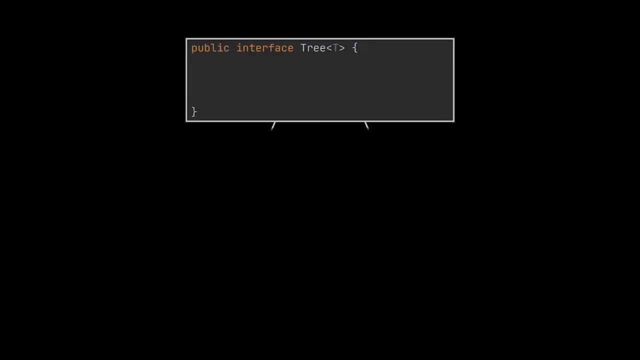 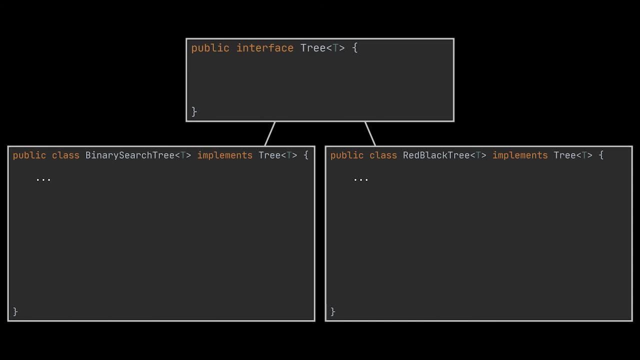 But instead retrieve them from collections. this way, we make sure that the iterator we are using is compatible with that particular collection. So what we should have had is a tree interface that is implemented by a binary search tree class and a red-black tree class. 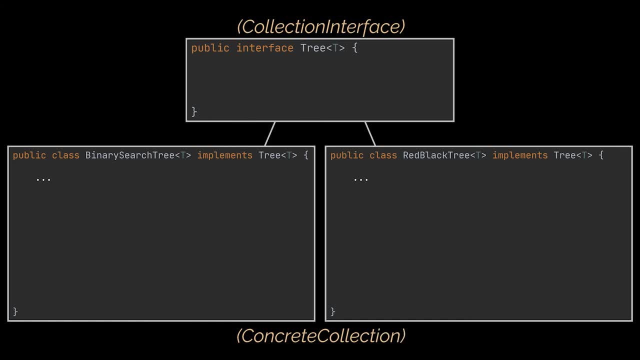 The tree here is the collection interface, And the binary search tree and the red-black tree classes are the concrete collections. The collection interface declares one or multiple methods for getting to a specific collection iterators that are compatible with the collection in question, whereas the concrete collections